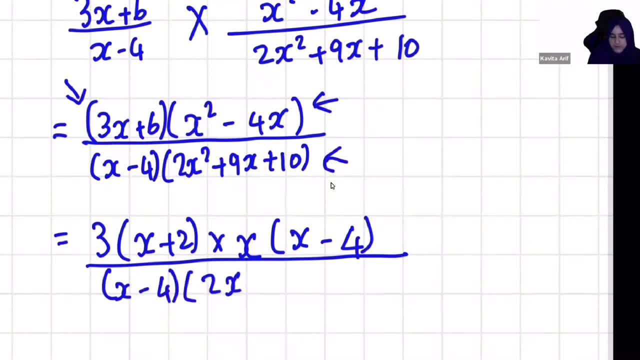 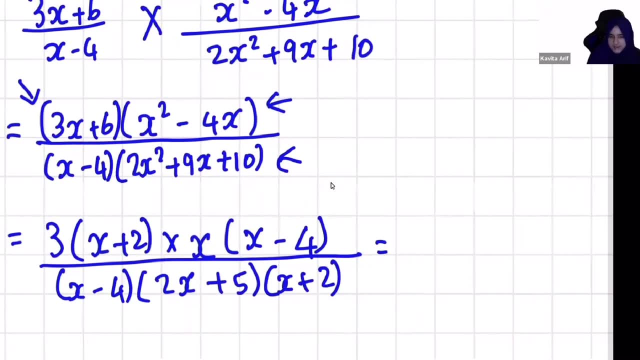 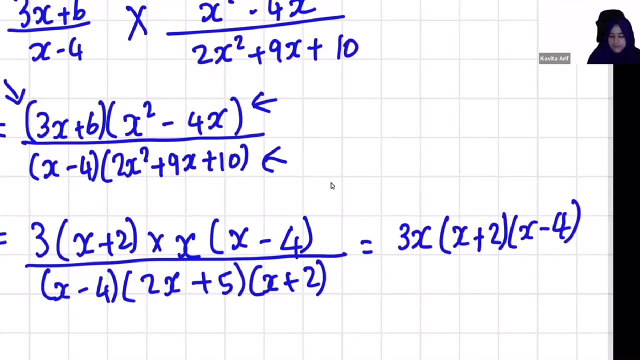 And then I've got placing this one into brackets: 2x plus 5, x plus 2.. Okay, and then I'm going to start over, so I'm going to rewrite it as 3x x plus 2, x minus 4, over x minus 4,. 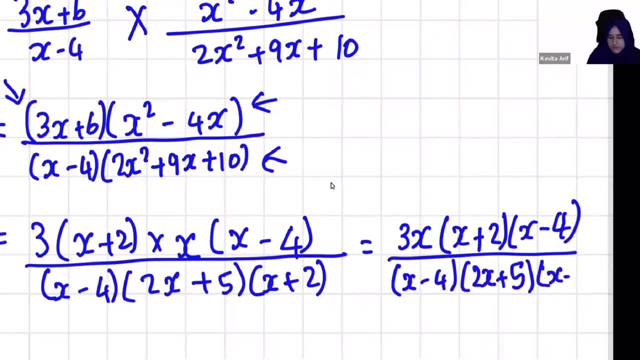 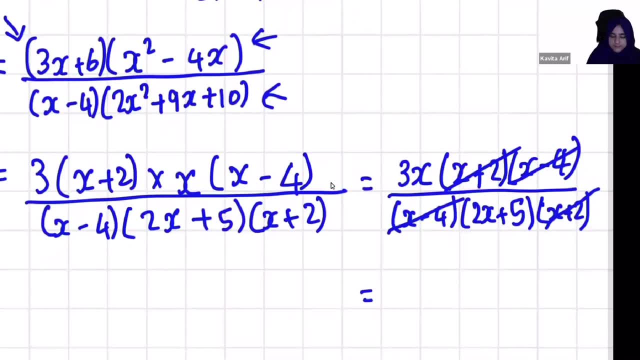 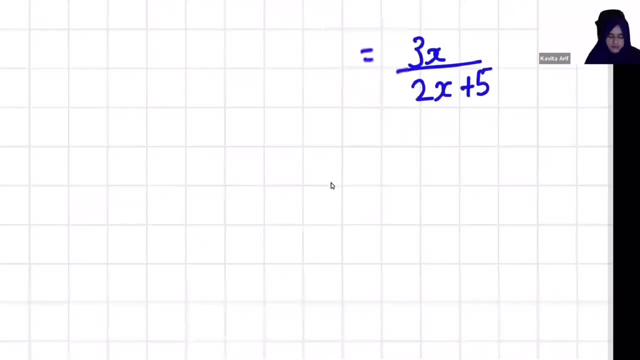 2x plus 5, x plus 2.. Cross this out. this is x plus 2 now, So the answer will just be 2x plus 5, x plus 2.. 3x over 2x plus 5.. There we go Now. the next question I'm going to do is similar, So I'm 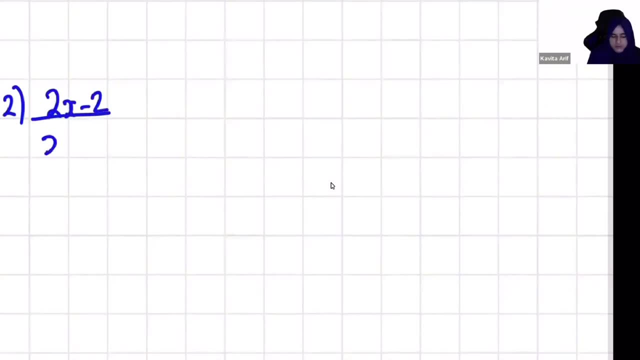 just going to do 2x minus 2, over x plus 5, divided by x squared minus 4x plus 3, over 2x squared plus 13x. So okay, and factor away is the first Numerate, that, and then 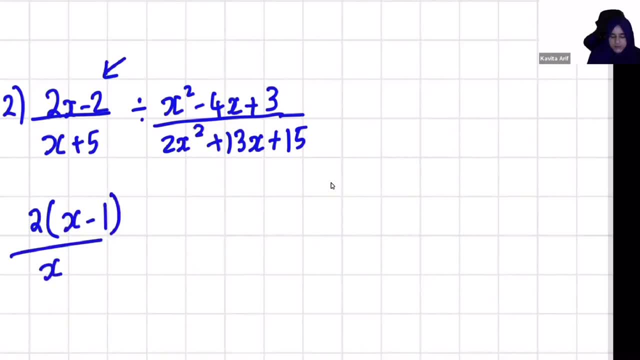 I'm going to do this in the numerator, So that's 2x minus 1, over x plus 5.. So I'm going to use the kfc methods of my times and flip the second fraction over 13x plus 15, over. 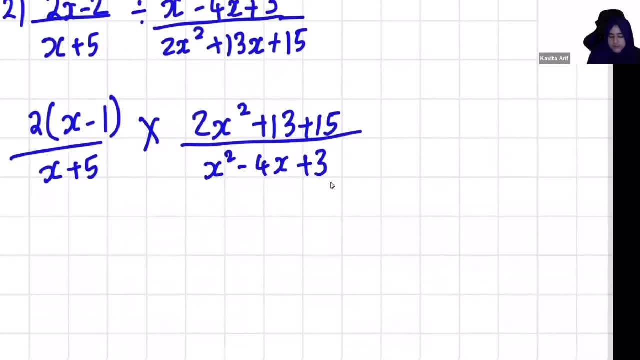 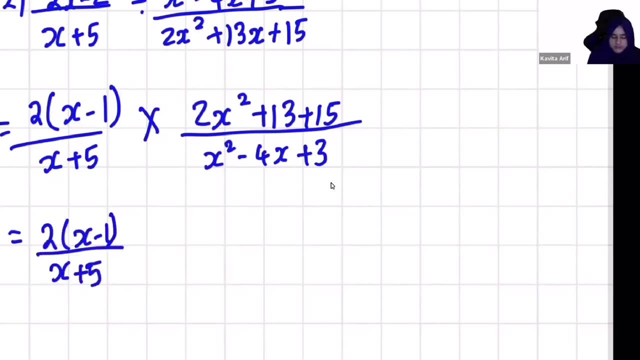 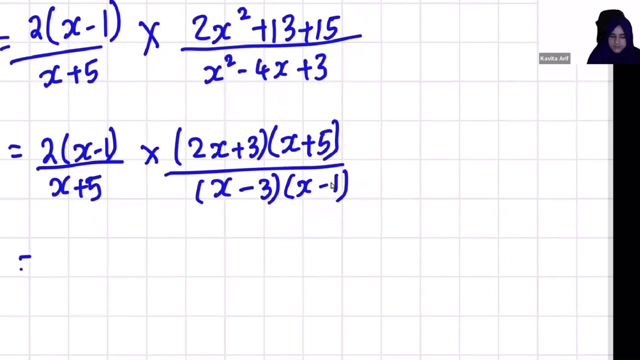 2x plus 4, x plus 3.. I'm going to factorise So 2x minus 1, x plus 5.. There we go, x plus. Then we can factorise the numerator like this: by the numerators we get 2x-1, 2x-3, x-5. 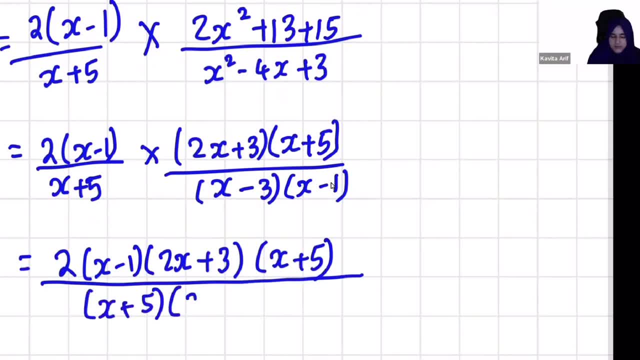 over x-5, x-3, x-4.. So now we can see what's in the numerator and denominator, as we can see Like this, and then we get 2x-2, x-3 over x-5. x-3 is the answer. 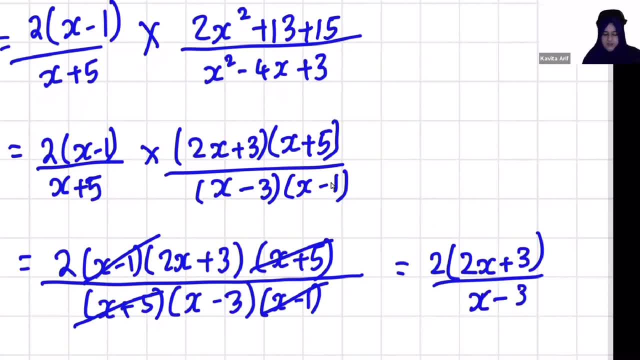 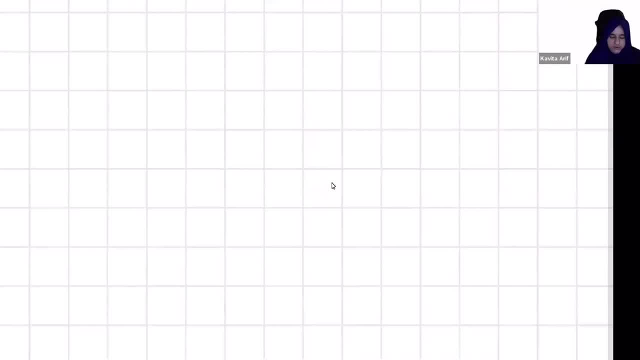 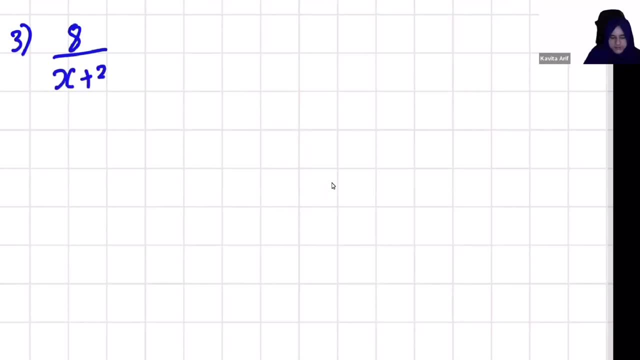 There we go Right. we'll have a go at another question. It's going to be a little bit more harder, So we'll start with the numerator. So we've got 8 over x-3 plus 3x-8.. 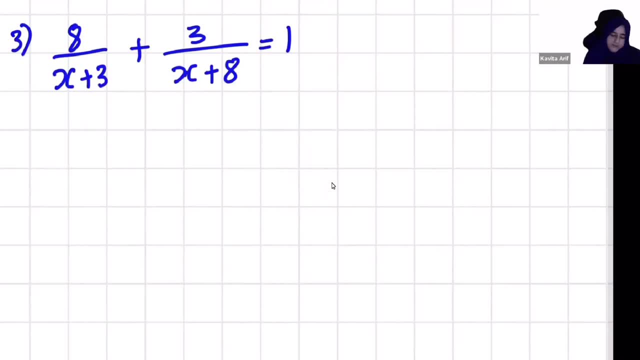 This is equal to 1.. We need a common denominator. so the first denominator we're going to multiply by x is 8.. And we're going to multiply the denominator numerator by this And x plus 3 for the second. Then we'll rewrite it. 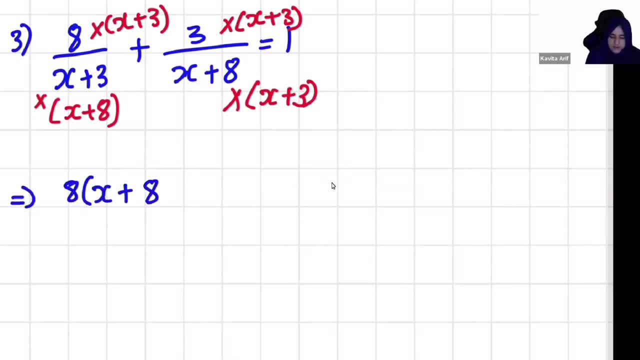 So we'll get 8x plus 8.. Okay, and then we're going to have x plus 3, x plus 8 in the denominator Plus 3x plus 3 over x plus 3, x plus 8.. 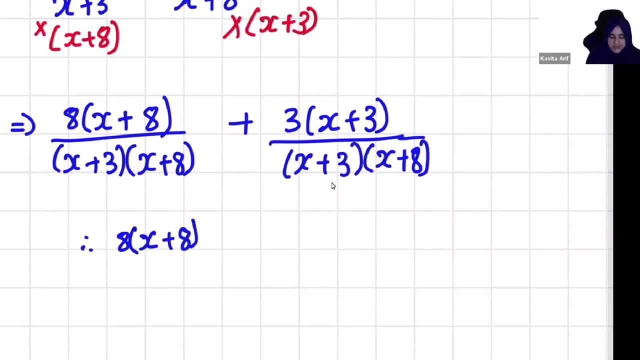 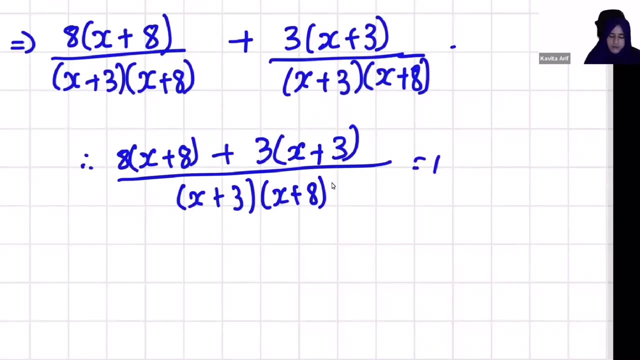 And from here, plus 3x, plus 3,, 3.. And then we have this over: x plus 3,, x plus 8.. Okay, It's equal to 1. this There we go. all is equal to 1.. 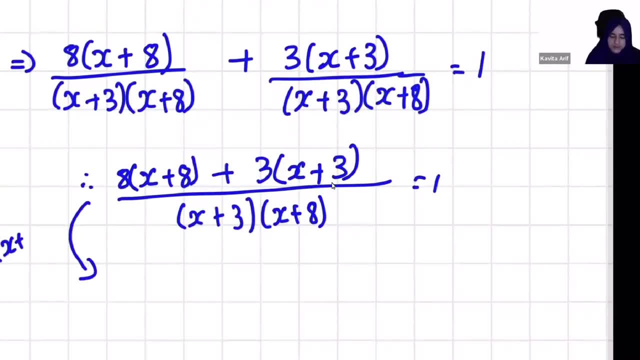 We're going to multiply both sides by x plus 3, x plus 8 times x plus 3, x plus 8.. So I'm going to end up with 8x plus 8 plus 3x plus 3 is equal to x plus 3, x plus 8.. 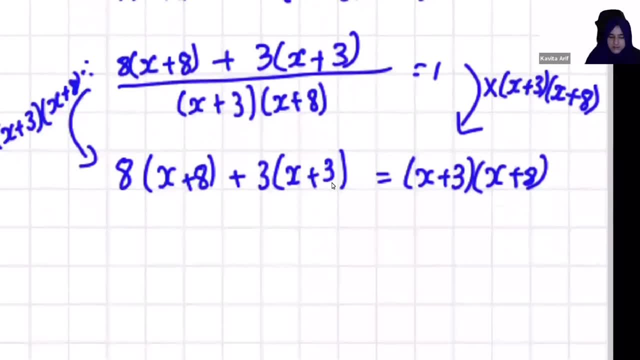 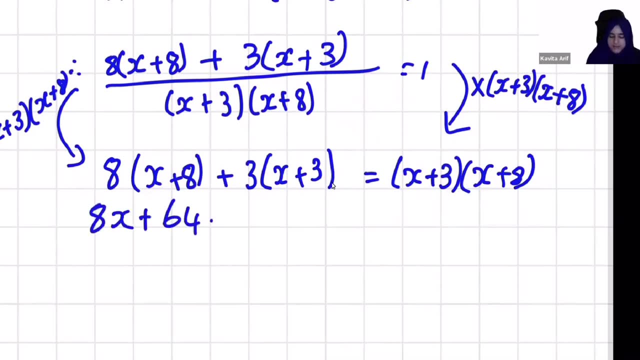 So what I'm going to do is expand all the brackets on both sides, And that was a big task. Okay, so we're going to have 8x plus 64 plus 3x plus 9 is equal to x squared plus, we get 11x plus 24.. 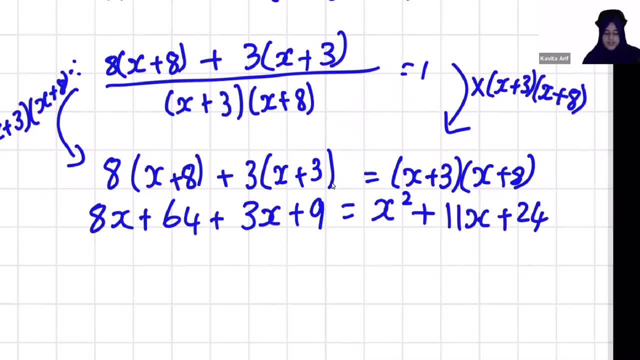 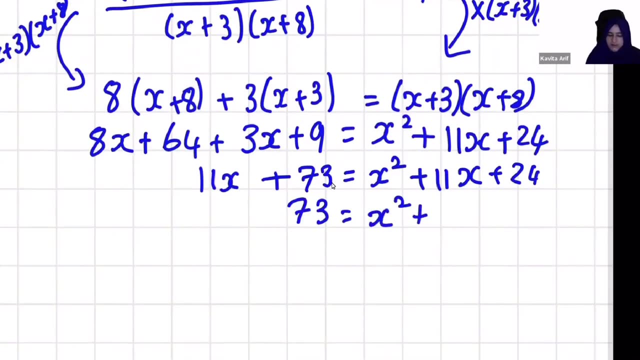 There we go, And then we can simplify and we get: 11x plus 73 is equal to x squared plus 11x. And then we can still simplify again further. So we get: 73 is equal to x squared plus 24.. 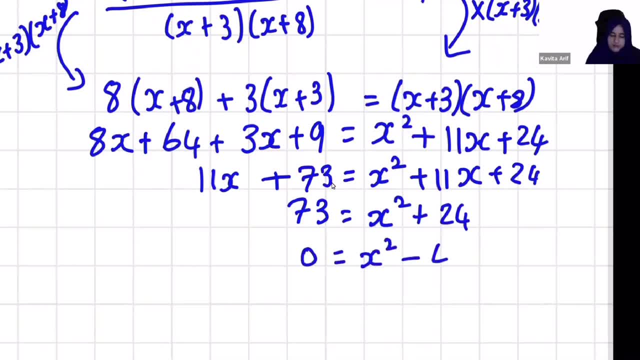 So then we get: 0 is equal to x squared minus 49.. And therefore x is equal to minus 7 or x is equal to 7.. There we go, So that is your solution. Thank you for watching. Stay tuned for more videos.